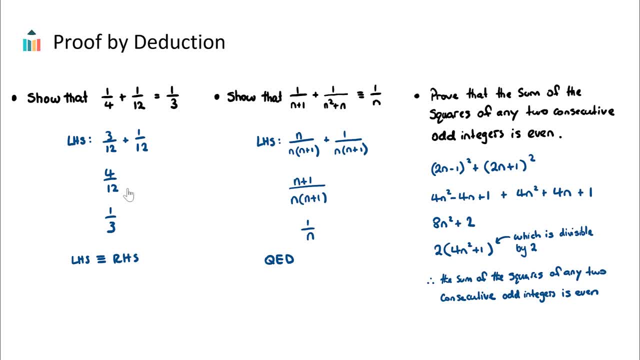 numerators, which is 4 over 12.. Now, 4 over 12, we know we can simplify that to be 1 over 3, and 1 over 3 is now our left-hand side, which was our right-hand side. So we have showed that this. 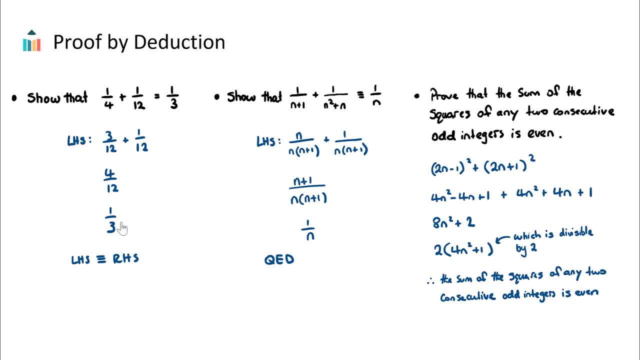 left-hand side equals the right-hand side. and once you get to this step here in your proof, what you can do, you have two options. You can say, well, the left-hand side is equivalent to the right-hand side, or alternatively, you can put this statement here: QED, You can put it right. 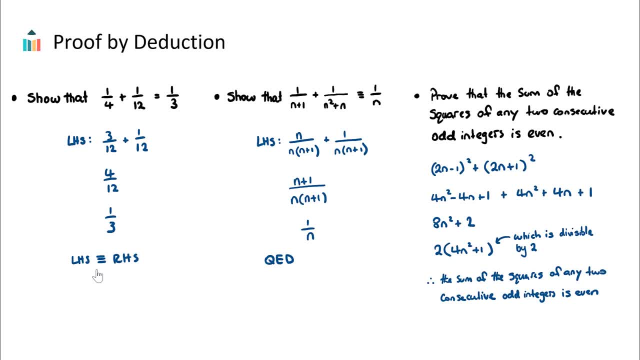 here and QED. it's a Latin phrase and it means well which, what was to be demonstrated or what was to be shown. We have shown that the left-hand side equals the right-hand side. Okay, so, once we've transformed one side to equal the other side, and in this, 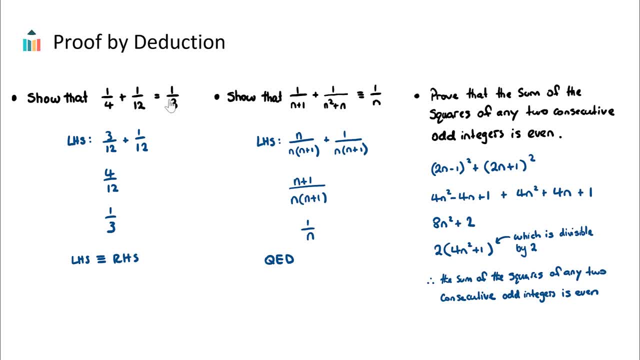 question here. we've transformed the left-hand side to equal the right-hand side, but you can choose. if this maybe this equation was flipped and the one-third was on the left-hand side and these two terms were on the right-hand side. you can transform the right-hand side. 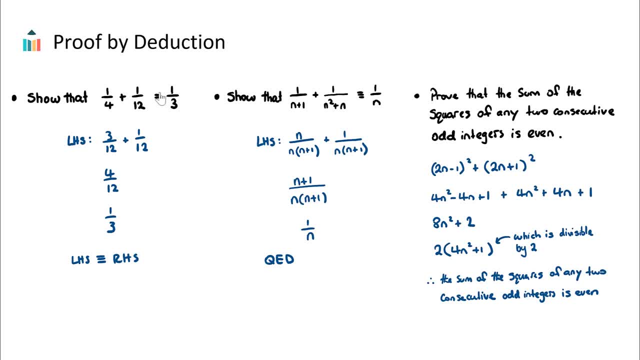 to be equal to the left-hand side. So either or is fine, but we can't move things across the equal sign in these types of questions. That's a rule that we can't break. Okay, so that's the first one done. Now. the second one is quite similar. What we have here is: we want 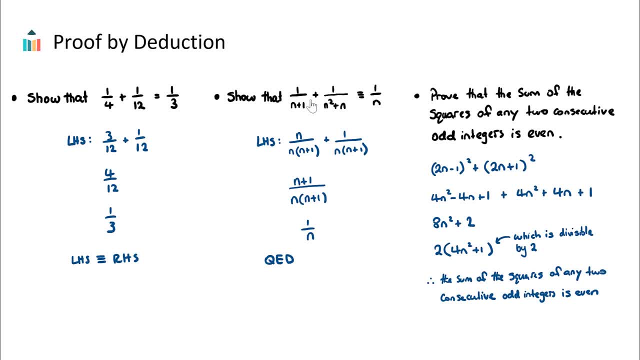 to show that 1 over n plus 1, plus 1 over n, squared plus n, is equivalent- this is our identity symbol- to 1 over n. Okay, so let's look at the left-hand side here, because this is what we need to. 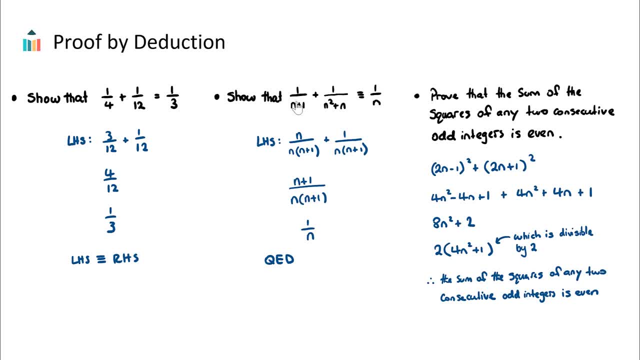 transform to equal the right-hand side. We can multiply top and bottom by this fraction, here by n, and we will get n over n times n plus 1, and then we are adding and on this, on the denominator of the second fraction, I've factored out the n to be n. 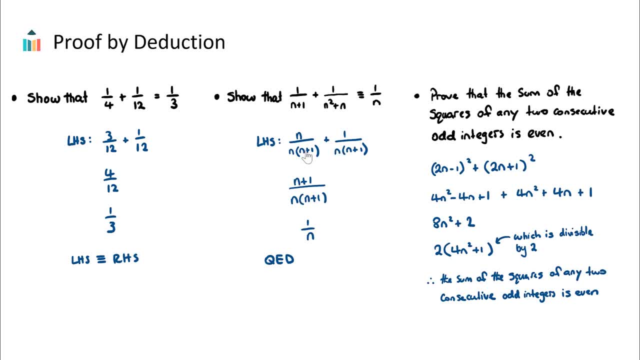 out the front of n plus 1, such that we have a common denominator here. Therefore, we now have n plus 1 over n times n plus 1.. The n plus 1's can cancel out and we will simply be left with 1 over n, which was the right-hand side. So as, as we said earlier, we 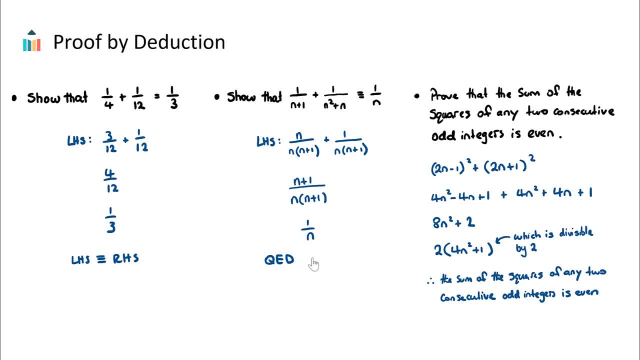 can either put left-hand side is equivalent to the right-hand side as our concluding statement, or you can put QED: Okay, the last one's a bit of an extension on from the basic proof by deduction questions. a bit of a worded question here, so let's go through the question. 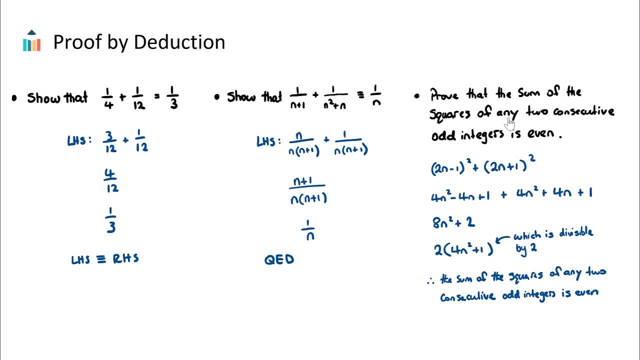 It says, to prove that the sum of the squares of any two consecutive odd integers is even Okay. so let's firstly try and define some things here. Well, two consecutive odd integers, that can just be 2n minus 1 and 2n plus 1, because let's just say n is some, is any number. 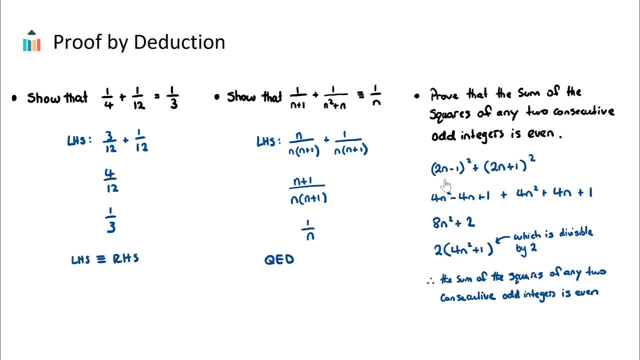 If we say: well, 2n is just 2 times that number. we know that 2 times any number is an even number. I multiply anything by 2, I get to an even number. and then if I subtract 1,, 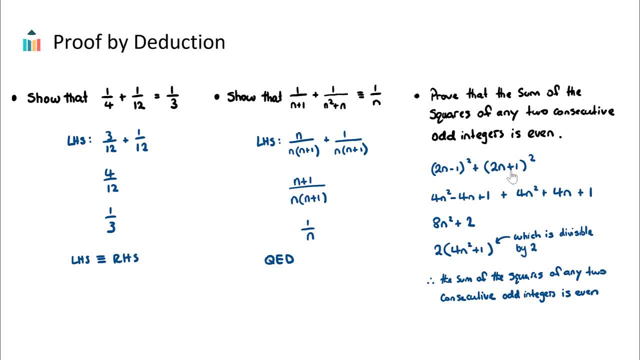 I get to an odd number And then if, alternatively, I added 1, that would be the next odd number. So 2n minus 1 and 2n plus 1, I have defined as my 2n plus 1.. 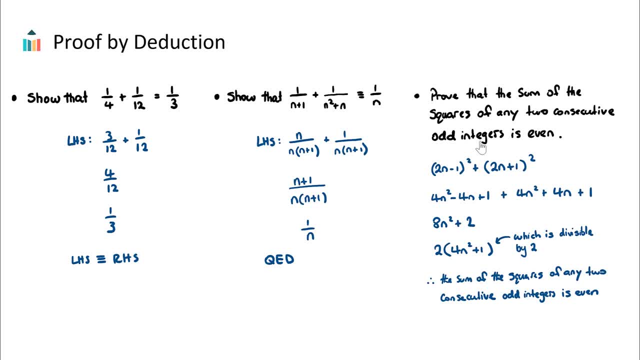 So I've got two consecutive odd integers and then if I want to prove that the sum of these two numbers, the squares of these two numbers, is even, well, I can start with this right here. I can then try and prove that this is even by expanding our brackets and 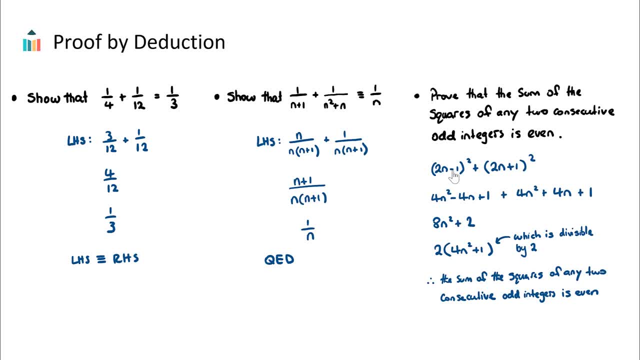 squaring both of these terms. So this will be 4n squared minus 4n plus 1, if we just expand this bracket plus And then we have 4n squared minus 4n plus 1. And then what we can do is collect our luck terms. this will become 8n squared. 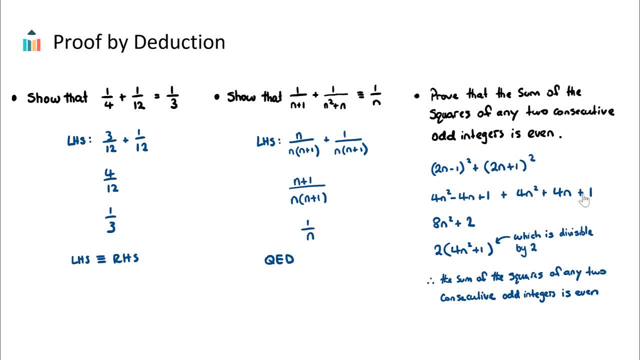 The negative 4n will cancel out with a positive 4n and we just have plus 2.. And then what we can do here is recognize that 2 is common. So if I factorize out the 2, I will have 2 at the front of 4n, squared plus 1.. 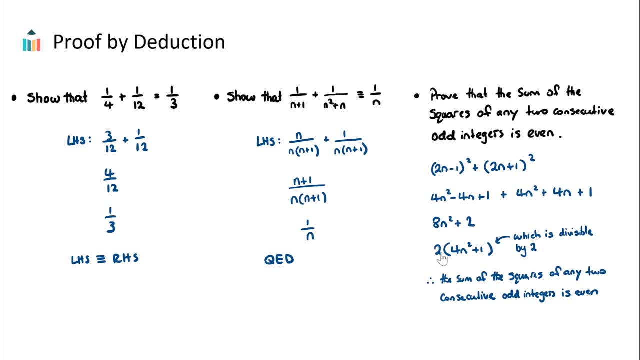 Now this here. I've simplified all the way down to this here. this here is currently the sum of 4n squared plus 1.. What I'm interested in is is this here? is this what I want to do? I want to show you. let's go back to that same example.